no gravity. In fact, if you built a skyscraper that was 200 miles tall and you were up on one of those top floors, you might weigh a tiny little bit less, but you'd probably weigh at least about 80% what you normally would. You're really not that much farther. 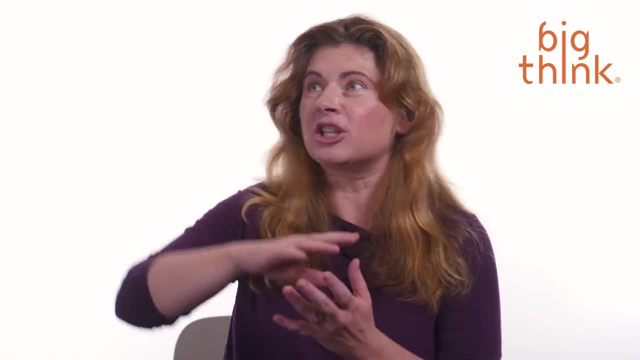 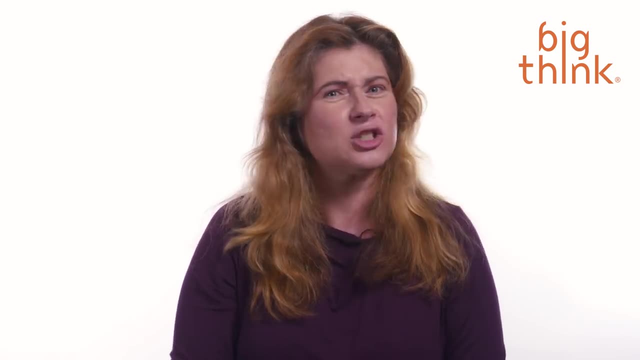 away from the Earth. So it's not that they're weightless because they're in space and far away from the Earth. They're actually close enough to the Earth to feel the gravitational pull of the Earth itself. So what's going on? Why are they floating around? Well, this: 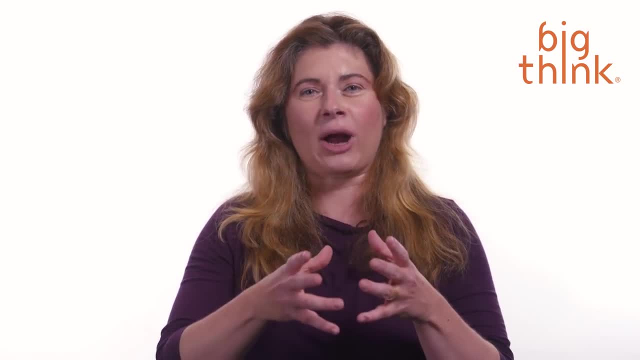 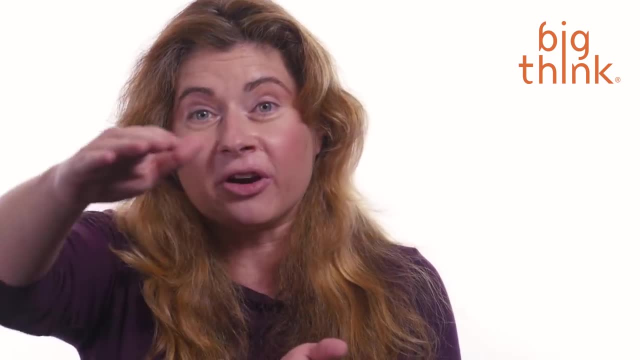 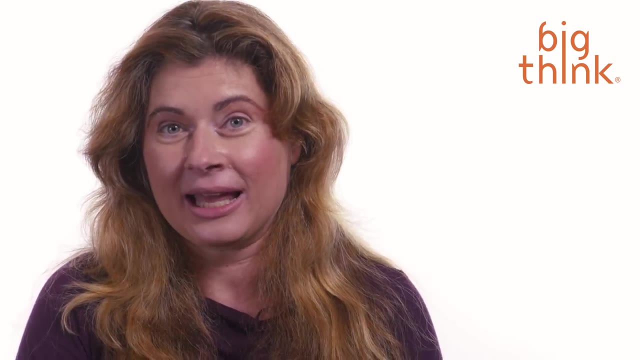 the rockets. Rockets launch spacecraft and get them going very, very fast, And if you're in orbit where the space station is, you're traveling at about 17,000 miles an hour. Now what happens to those astronauts is that they're going very, very fast, but they're 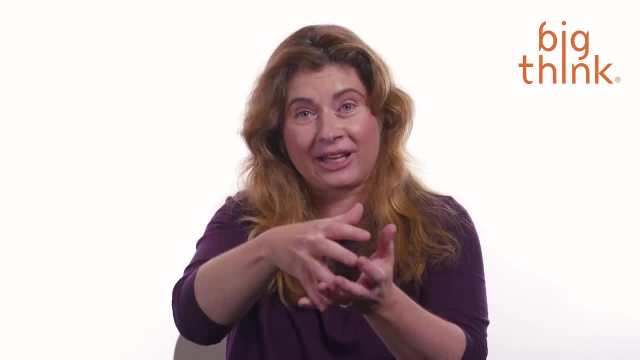 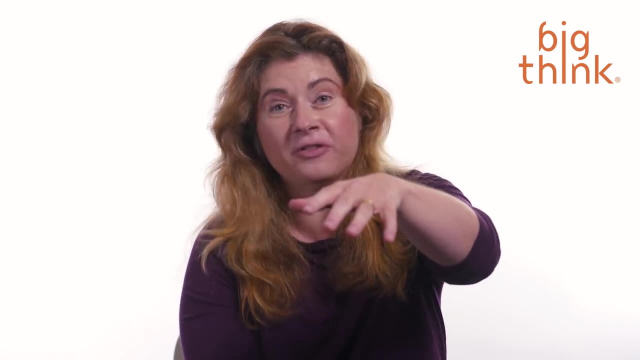 actually freely falling towards the Earth. The Earth has gravity and that gravity is pulling them down, just the same as what would happen as if you dropped a ball. If you dropped a ball, it would fall to the floor. The same thing is happening to the astronauts. They 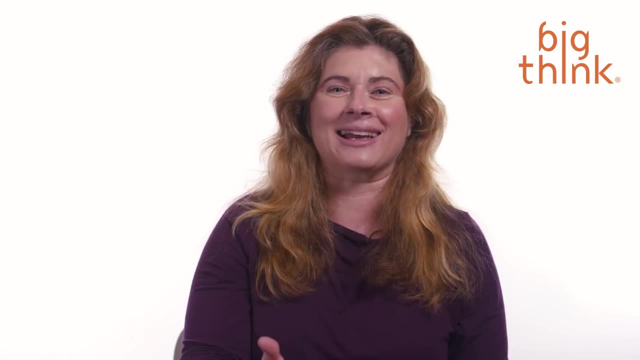 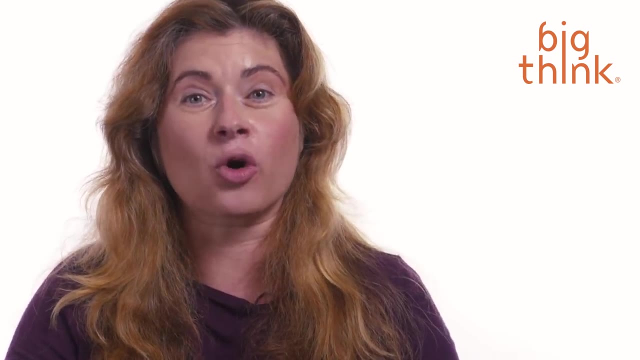 falling towards the surface of the Earth. But here's the cool thing: They're going so fast. they keep missing the Earth as they fall, And that's the definition of an orbit. Now, think about it this way: I talked about dropping a ball, The ball. 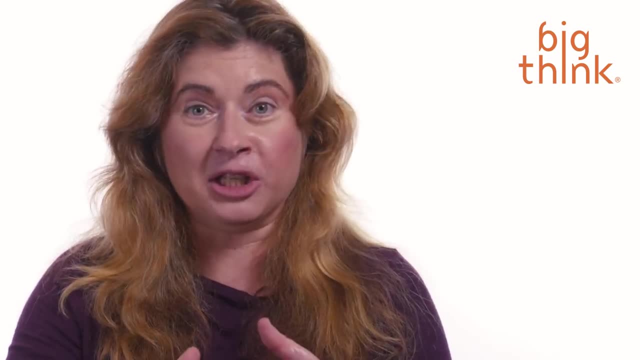 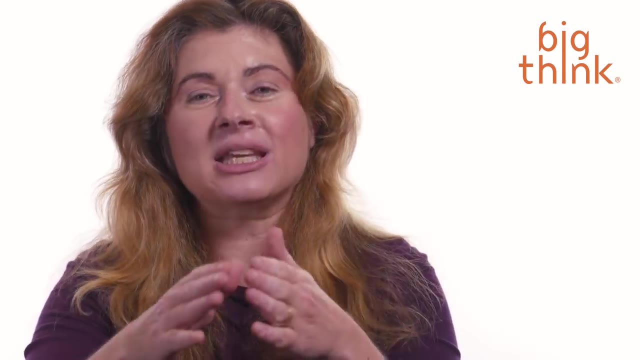 just falls straight down. What would happen if I put the ball in a little cannon and shot it out? The ball would start to drop towards the Earth the minute it left the cannon, But the cannon has given it some velocity, and so the ball might go a hundred yards. right, It might actually go a hundred yards before. 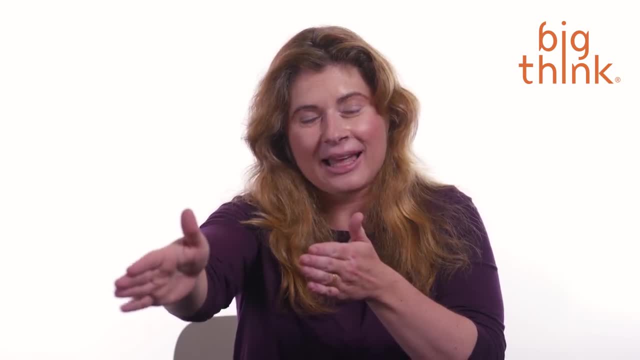 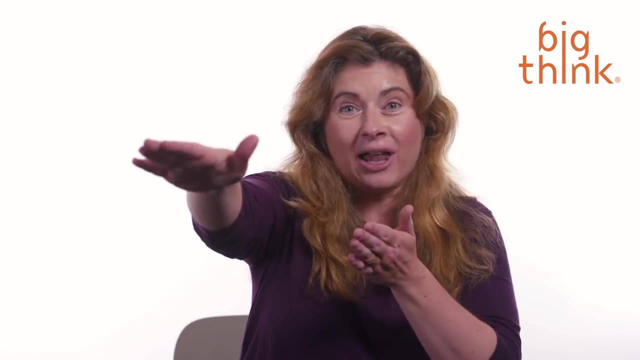 it fell because the cannon gave it that velocity. Now let's take an even bigger cannon, Let's take a huge cannon that can shoot things many, many miles. So you shoot the ball out. the ball is still falling freely towards the Earth. all the 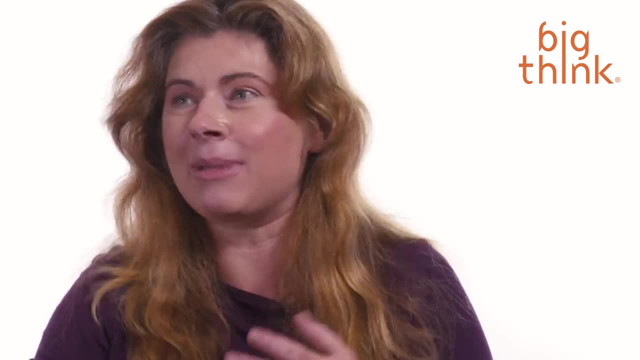 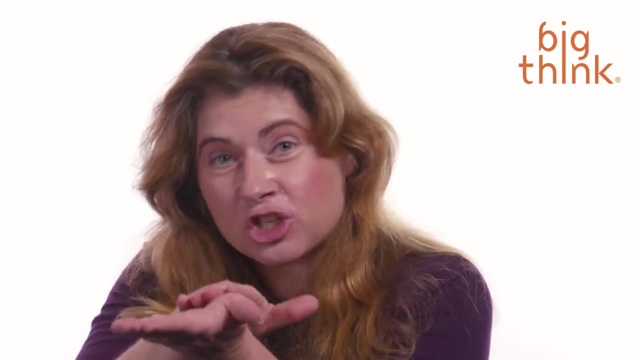 time. But now it goes farther because you've given it more velocity And maybe with a really big cannon you could shoot a ball a hundred miles. What about with a rocket? With a rocket, you could get something going so fast across the Earth that it would fall. And that's what we're going to do. We're going to go up to 17,000 miles an hour. that, as it fell freely towards Earth, Earth would keep curving away under it and it would keep missing it. That's what an orbit is, And that's why you need a rocket to get into orbit. You need to get yourself.